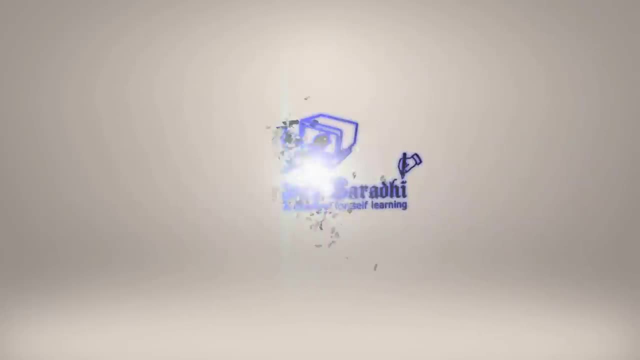 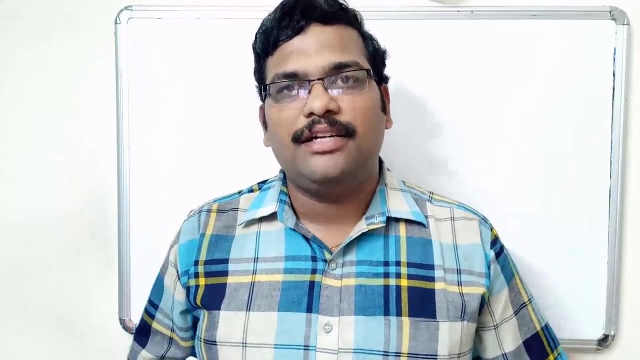 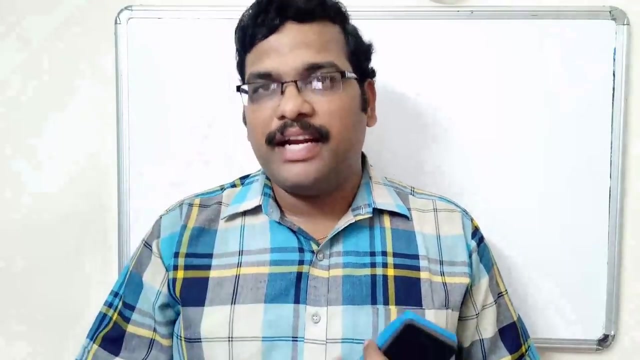 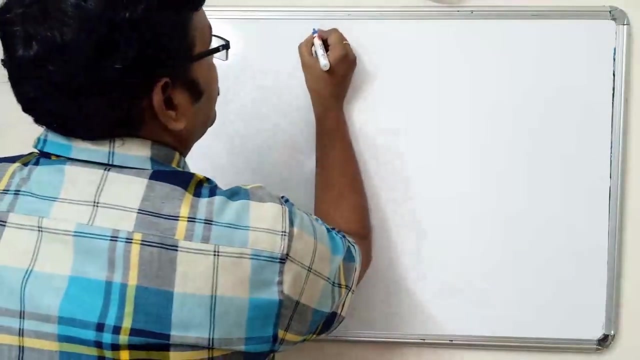 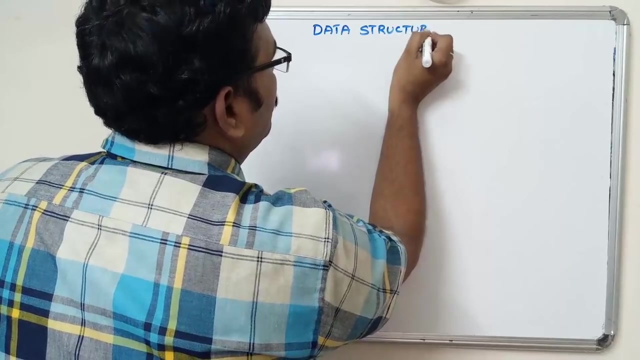 Hi friends. so from today I am planning to upload the videos on data structures. So in today's session we will see the introduction of a data structure. that means what is a data structure and what are the different concepts covered in the this? data structures, Right? so data structures- what is? 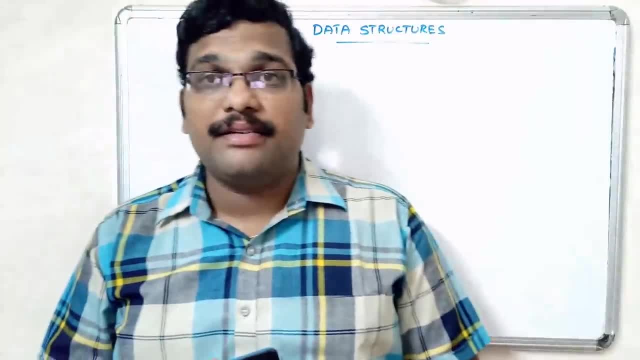 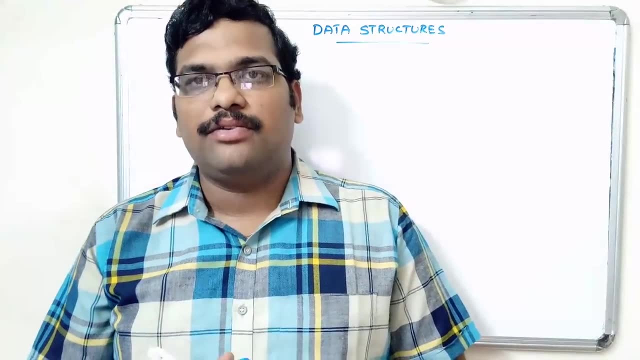 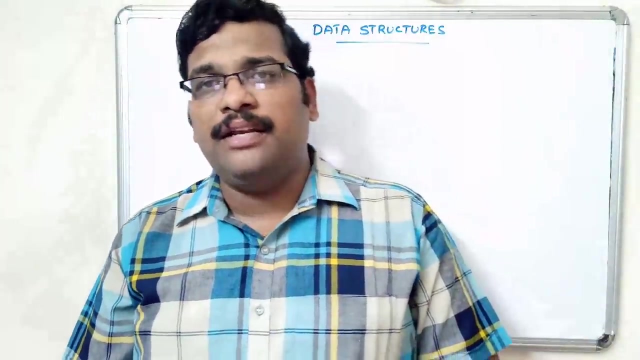 meant by a data structure. So the name itself indicates data structure. so that means organizing the data in the memory is called a data structure. So there are different ways to organize the data in the structure. So one example we have seen in the C language that is arrays. So 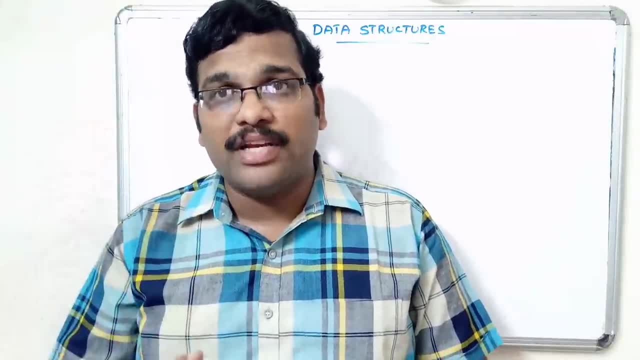 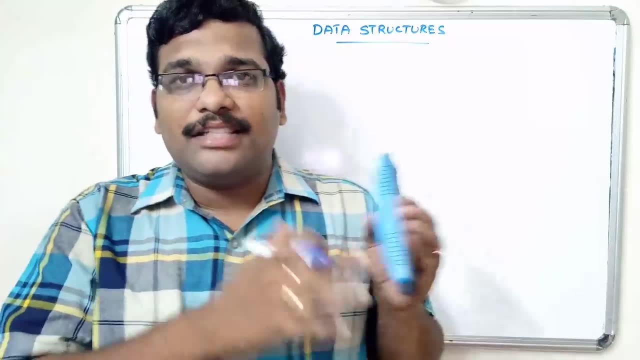 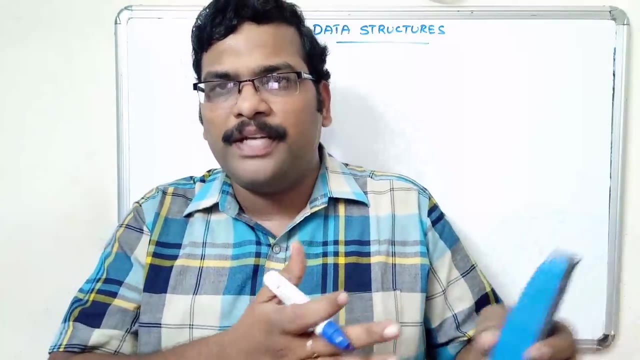 array is also a collection of elements. that means a collection of memory locations. So, because in the memory locations we are going to store the values. Right? so in that the structure of data is a sequential, that means one after another, Right, so it occupies the continuous memory. 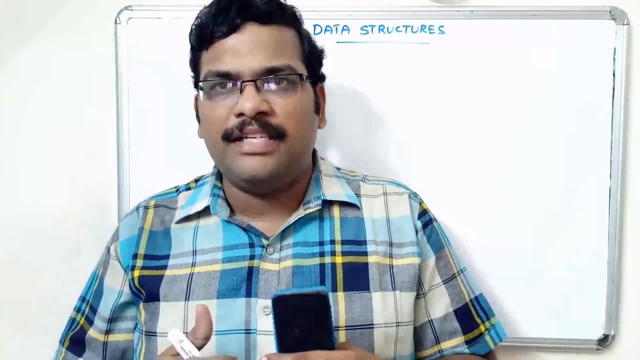 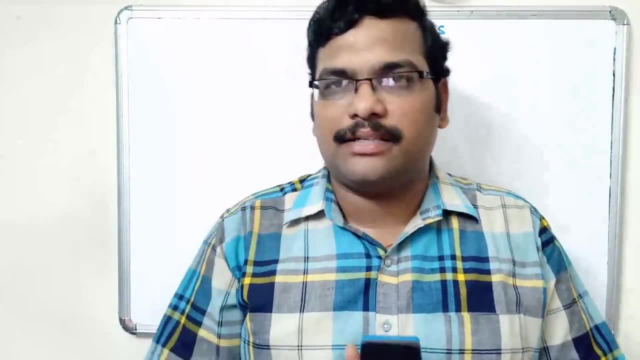 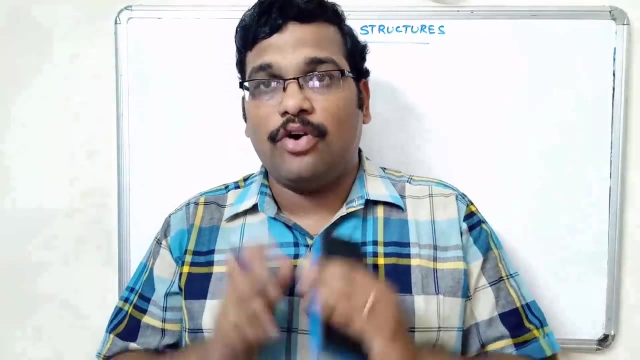 locations, So it is a collection of elements in that continuous memory locations. So that way the data is organized using the arrays data structure. So, finally, the definition of data structure means organizing the data in the memory location. So how many ways we can organize the data in the memory. 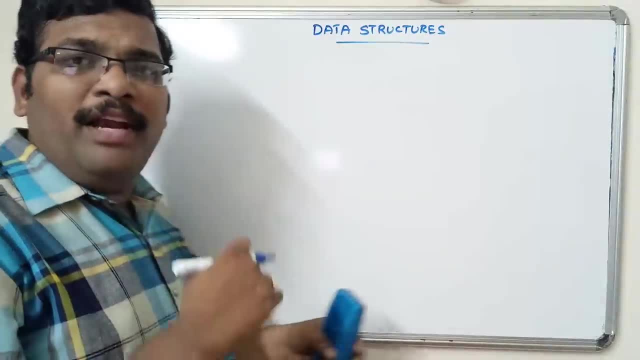 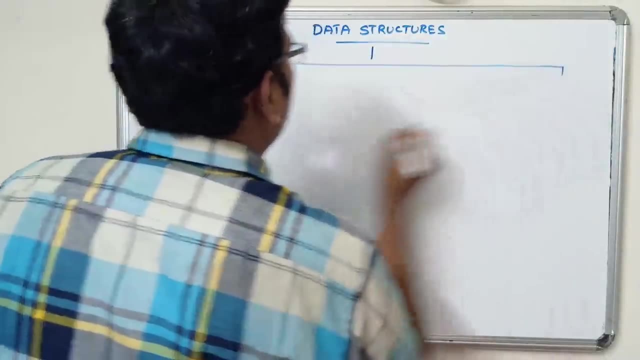 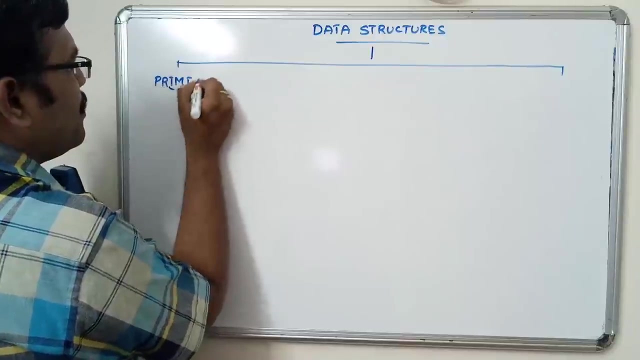 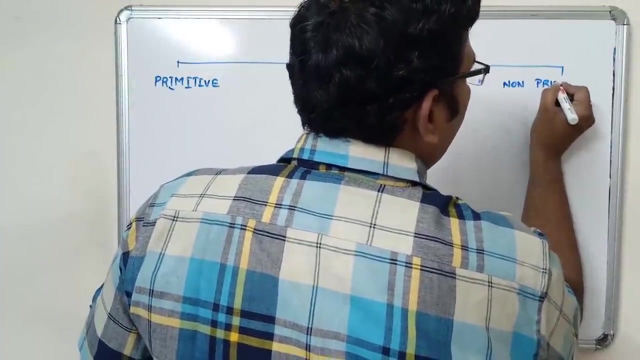 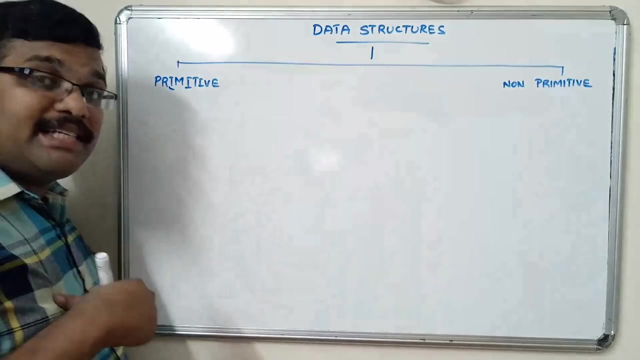 location. Right now let us see how many types of data structures. So there are two types of data structures. So one is primitive data structure and another one is non-primitive data structure: Primitive data structures and non-primitive data structures Coming to this primitive data. 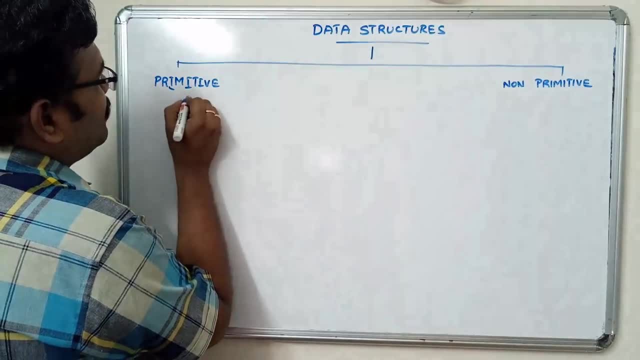 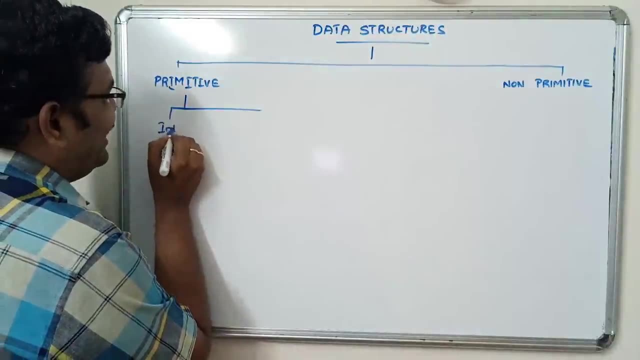 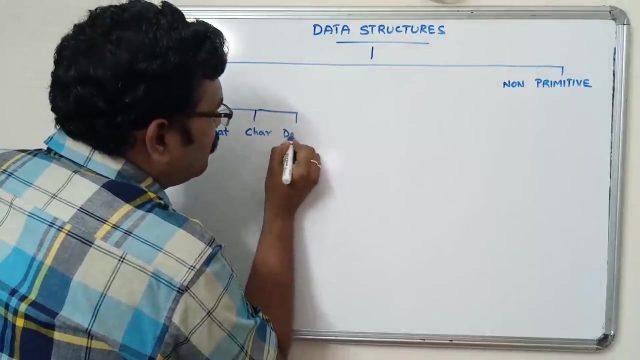 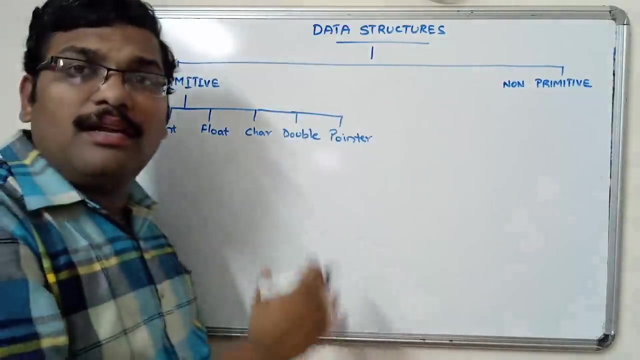 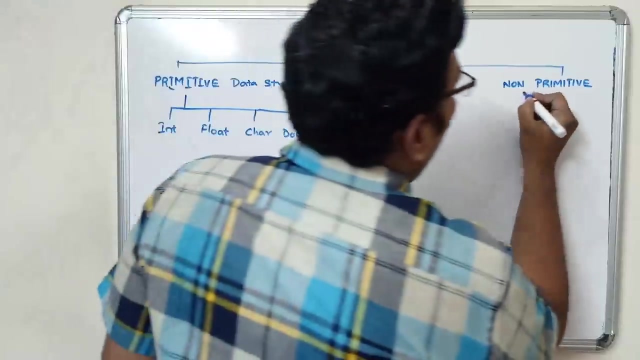 structures. we have already seen those data structures, See. so these primitive data structures are our primitive data types. Yes, so int, float, character, double and pointer. So all these comes under primitive data structure, Non primitive data structure. Now let us see how many. 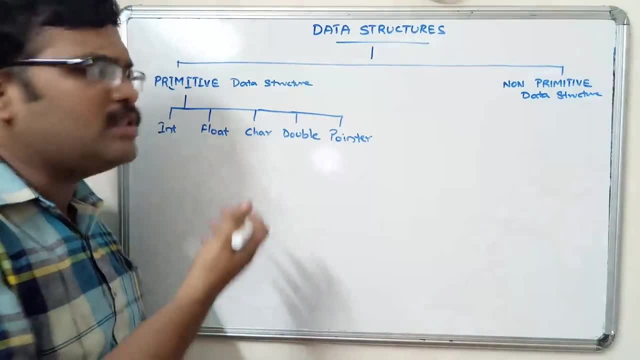 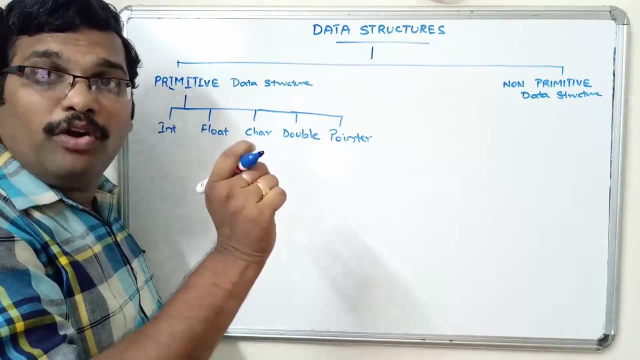 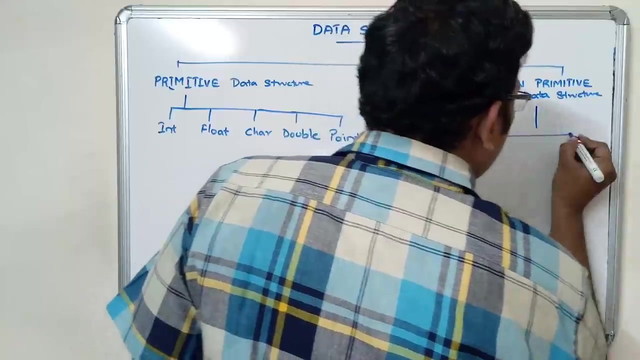 so these we have studied in C language. these we call them as primitive data types: right, integer, float, character, double and pointer. it's a single memory location which can hold the value only. next, coming to this non-primitive, it's again divided into two types, that is, linear data structures. 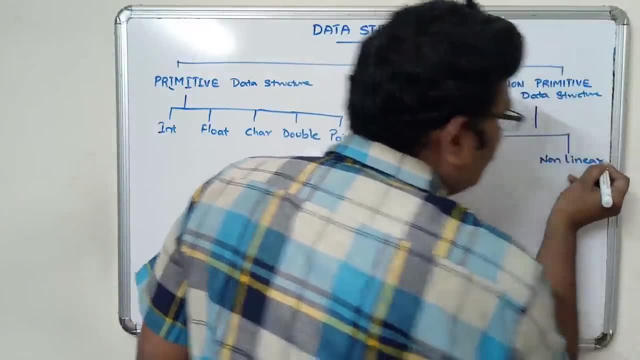 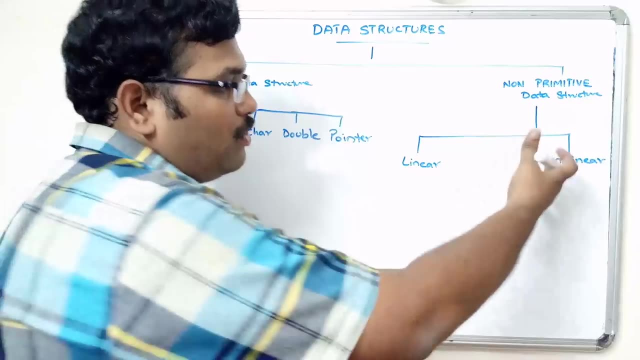 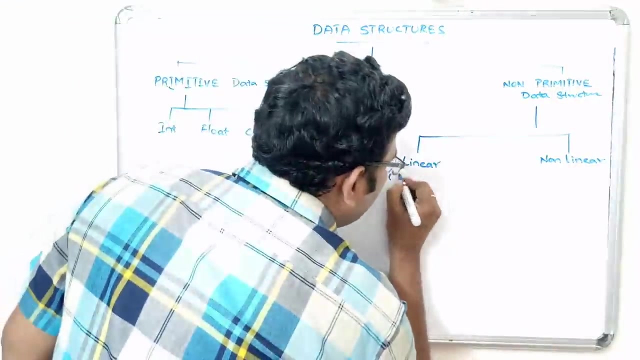 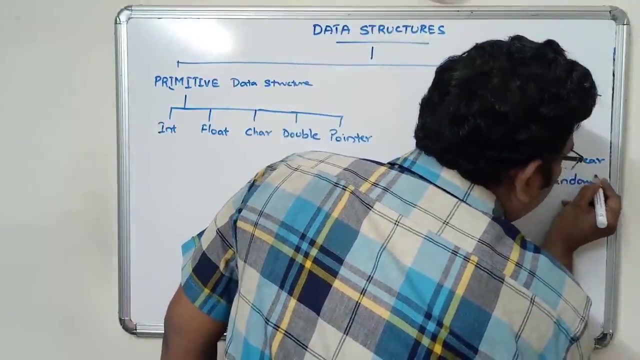 and nonlinear data structures. linear and nonlinear. so linear means a sequential, that is nothing but a sequential. so nonlinear, which is not a sequential, that we can call it as a random random. so this is a sequential, this is random. that means in this all the data will be arranged in sequential. 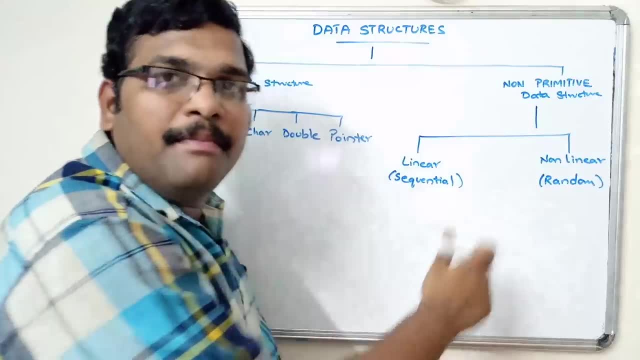 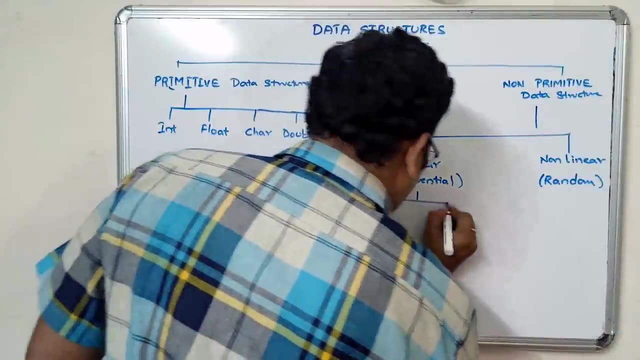 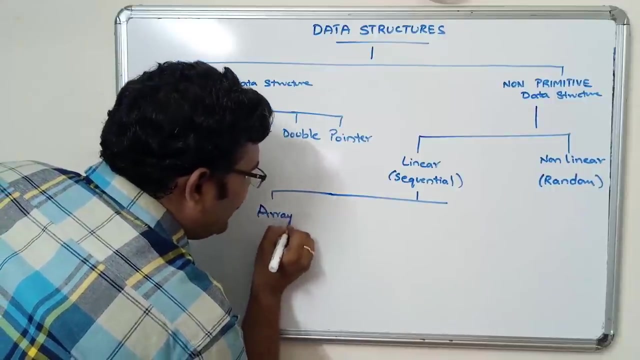 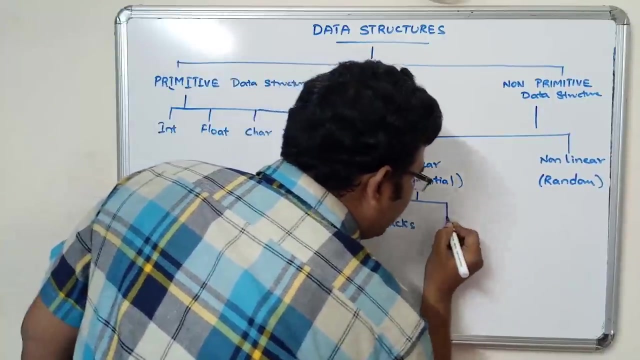 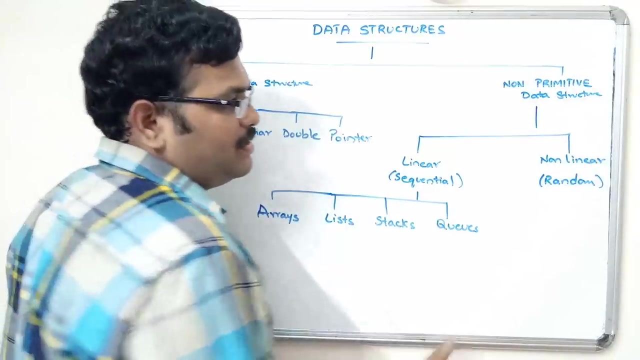 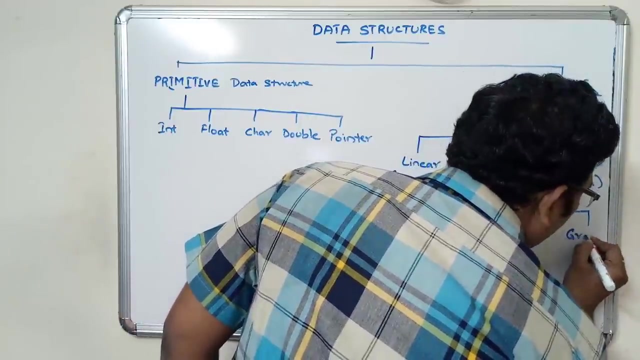 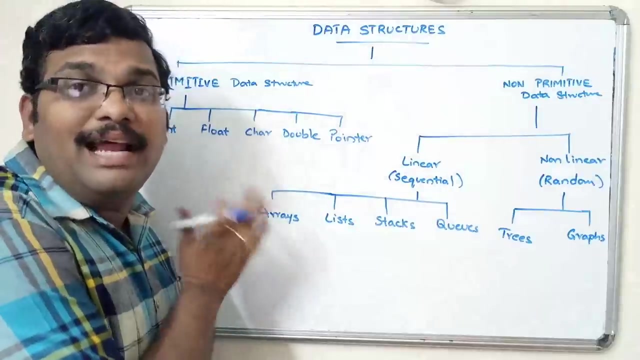 manner. here the data is arranged in random manner. now, what are the types of linear data structure? so first one is arrays, lists, stacks, queues. these four comes under linear data structure, nonlinear data structures. only two categories are there, one is a trees and graphs. trees and graphs, so again. so this we have seen in C language: arrays, the 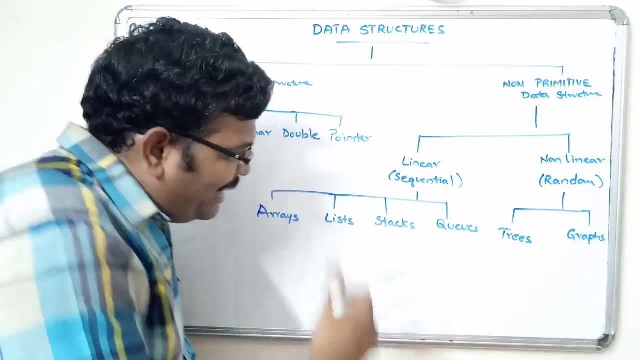 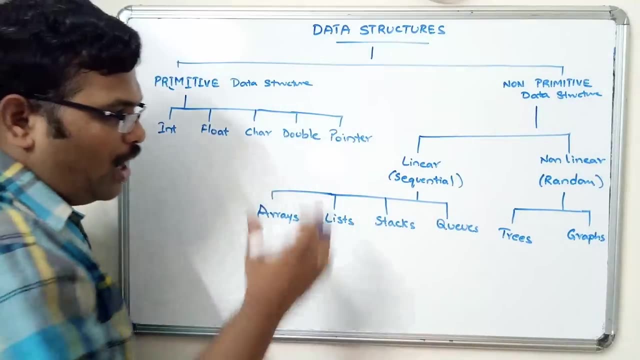 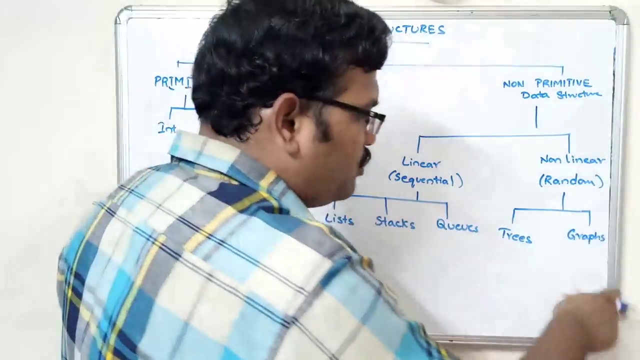 sequential elements. so now we have to see about the list, stack, queues, trees and graphs, so how the data is arranged in list, how the data is arranged in stack, how the data is organized in queues, how the data is organized in trees and similarly, graphs. so these are the 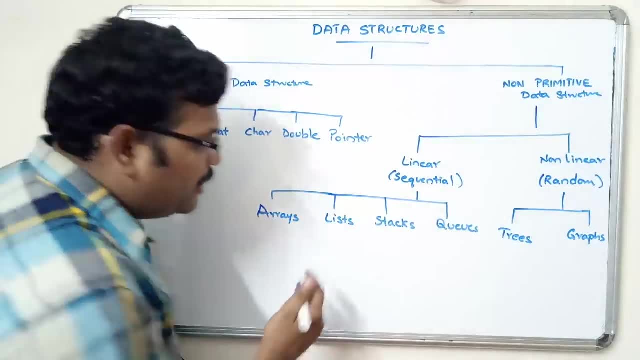 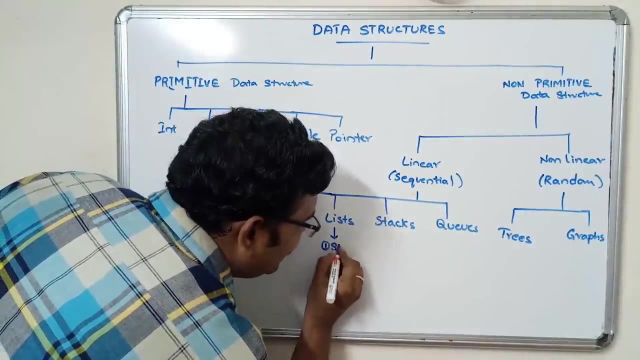 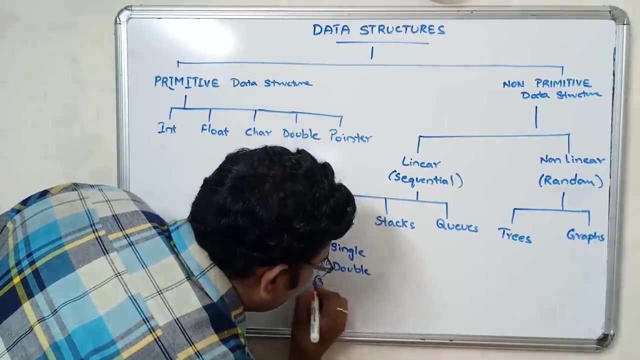 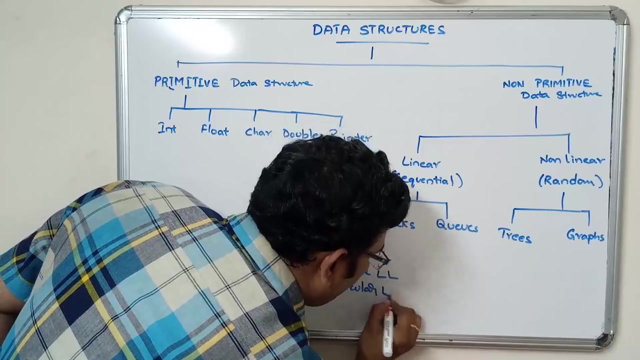 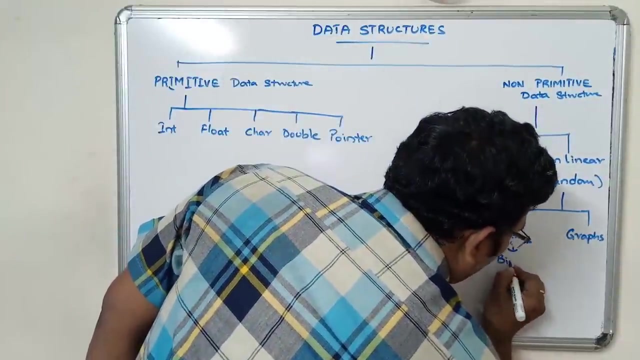 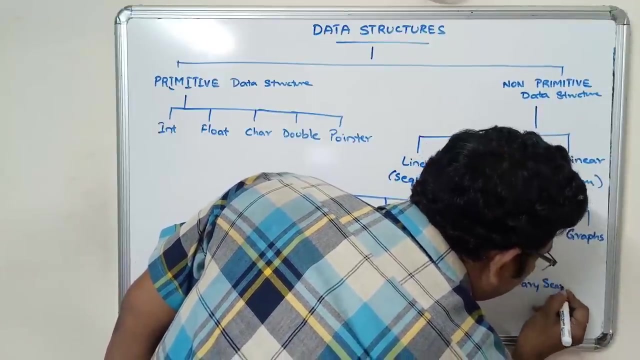 different types of data structures. right so in the list there are a number of categories, so under this one is single linked list. double linked list, circular linked list, elements linked list. right so here in trees we are going to discuss about binary trees, binary search trees, and there are a number of trees. right so? 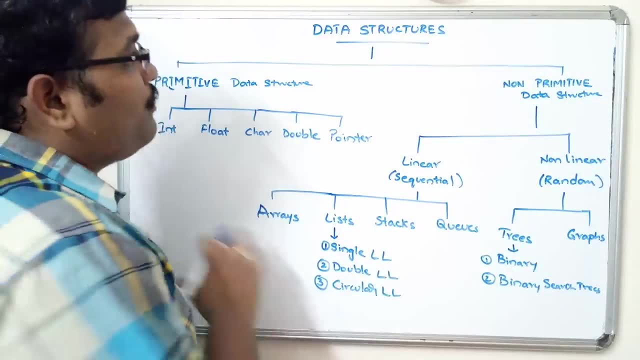 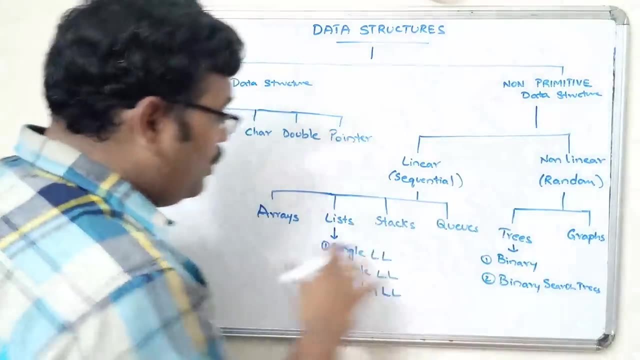 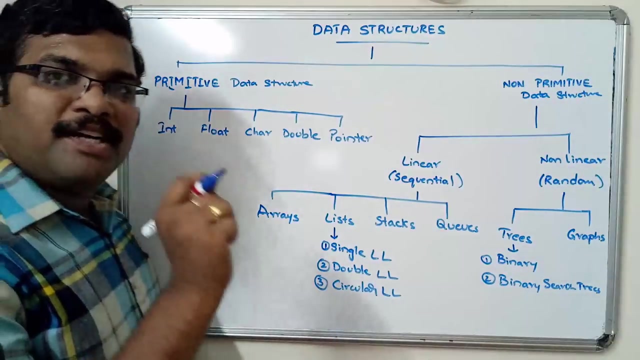 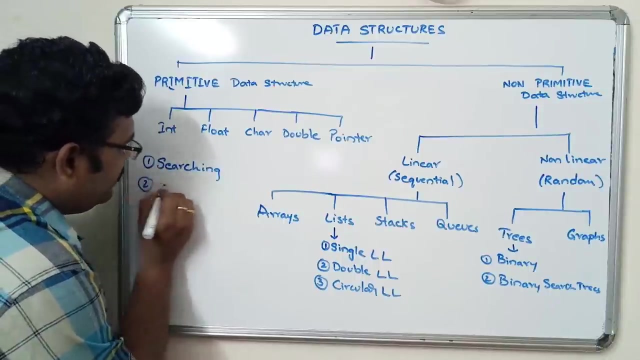 we will discuss in those sessions, right? so finally, the data structure interaction. is this thing so primitive and non primitive? right and now there are common operations can be performed on these data structures, operations that so the major operations which can be done is searching and sorting. so we can. 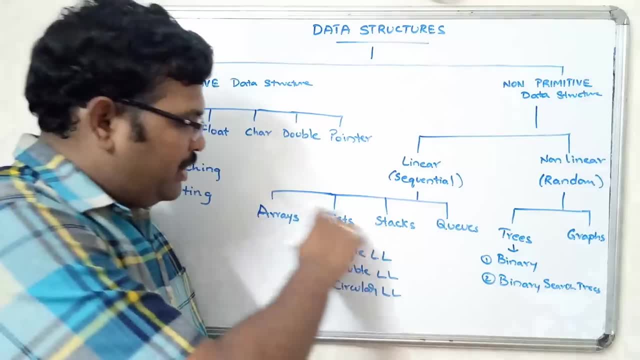 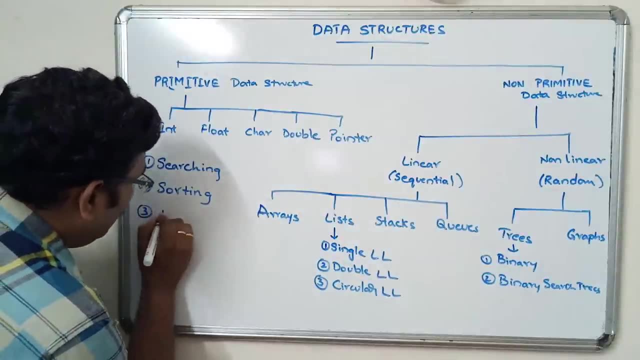 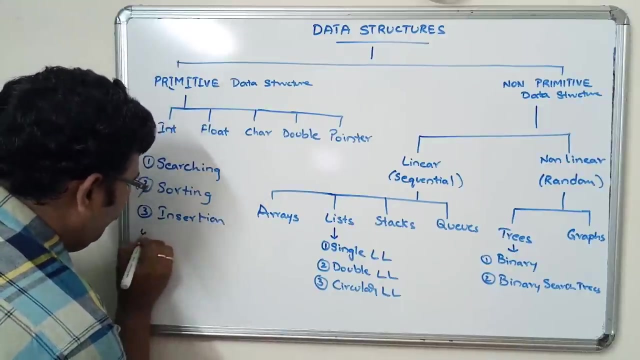 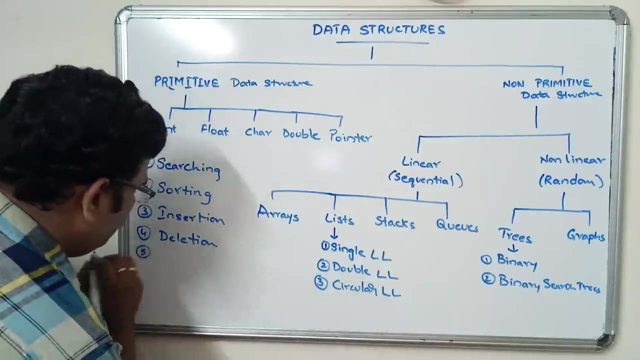 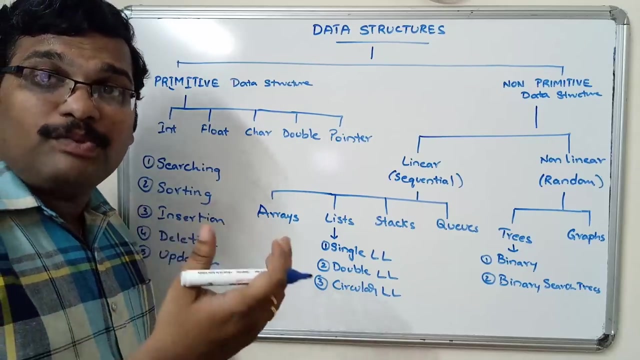 search an element in the data structure right. so in the in the list we can sort the elements and then see we can insert the new element right. insertion. similarly deletion, we can delete one element. next, updation, so we can update the elements. so that means we can replace one element with another element. 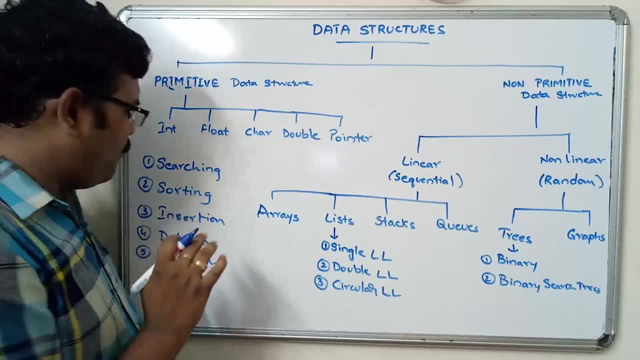 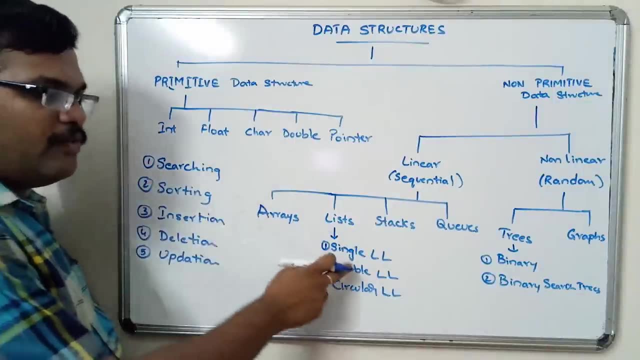 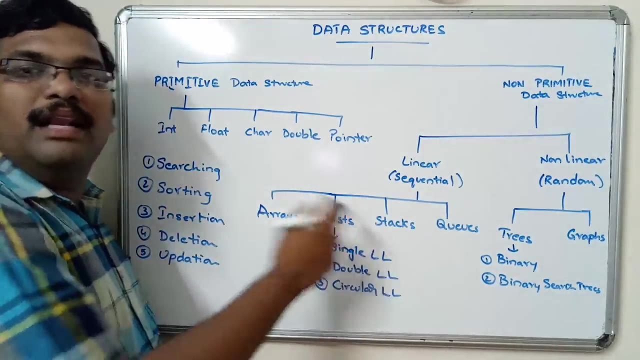 right. so these are the common operations to be performed in these data structures. so we can search an element in linked list, we can sort the elements of a linked list, we can insert an element into the linked list, we can delete the element from the linked list and we can update the element in the linked list. so 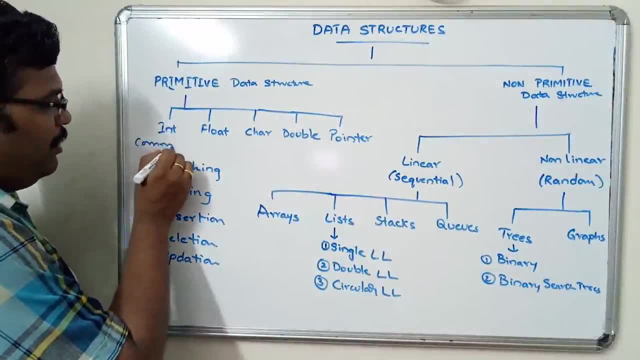 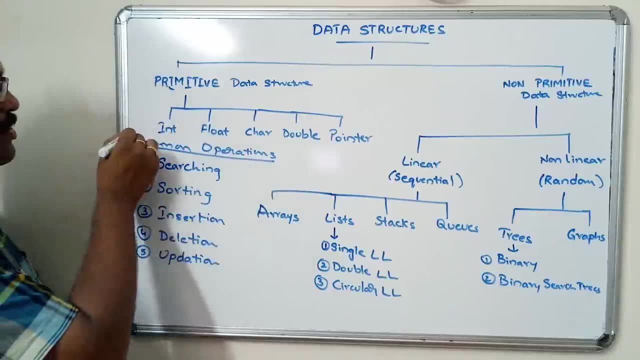 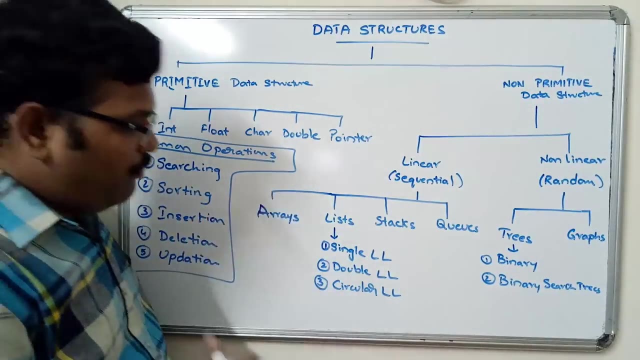 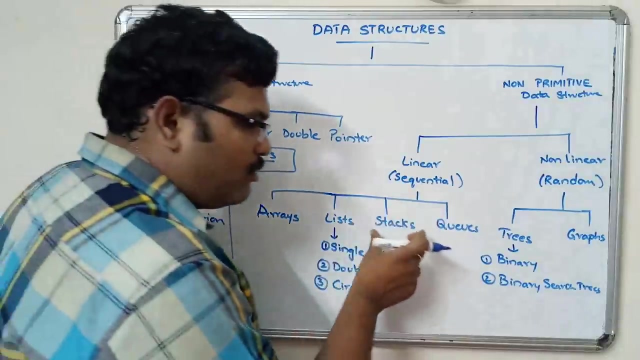 these are the common operations, so I will write here: common operations on data structures. so this is the common operations on data structures, right? so we are going to discuss about the list. in the list, we have to apply all these operations, and then we have to apply all these operations, and then we have to.